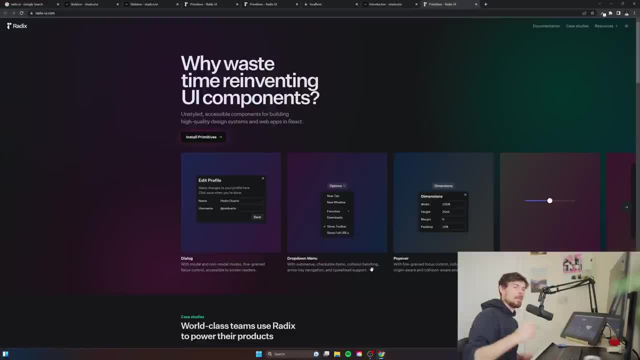 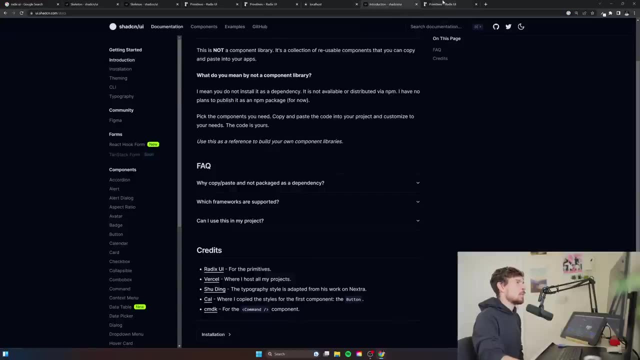 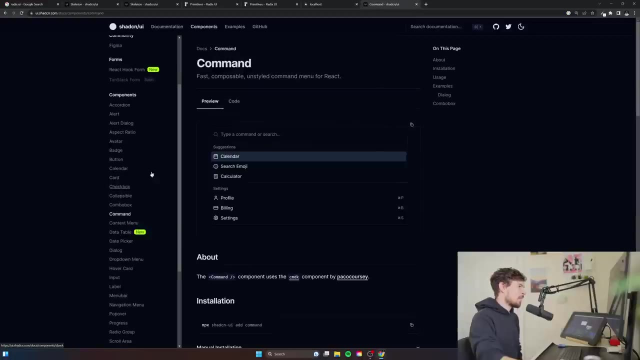 whatever you want with them, but they have the accessibility right. So when you're making forms, one of the most annoying thing is adding the accessibility to it. So chat CN was built on top of this, So what we're going to do is essentially create a. yeah, here are all the components. 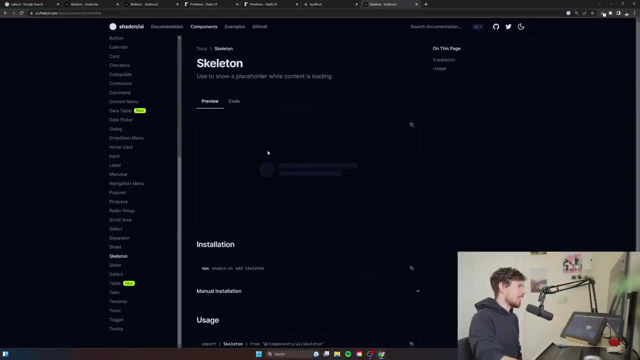 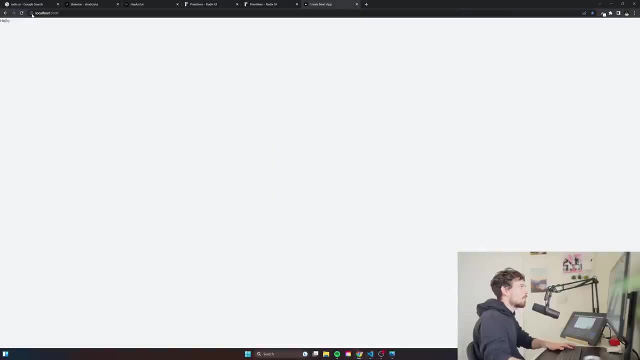 but we're just going to choose one for this episode. I'm going to go with skeleton and I'll show you perhaps one of the simplest ways you can do that. So I'm going to go with skeleton, So let's get going. Okay, cool. So here we go. So we just have a hello here And what we're going. 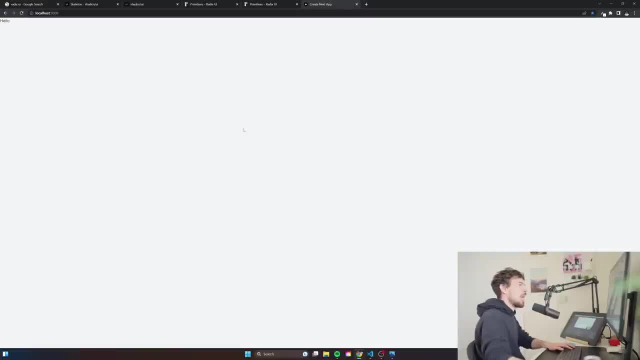 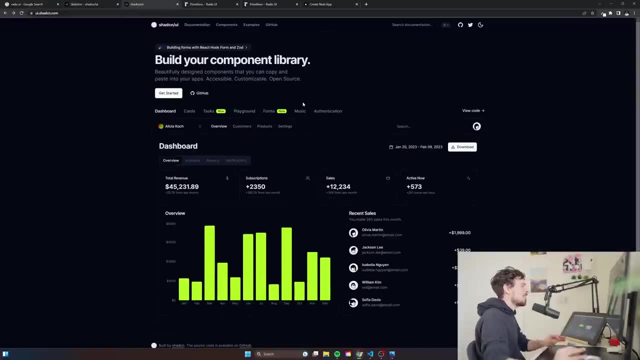 to do is we're going to fetch some games, And if the games are not loaded yet, then we're going to pop in a skeleton for us. So to get started now, you'd usually just not even have to install anything with chat CDN, because it was never intended to be used like that. It was intended. 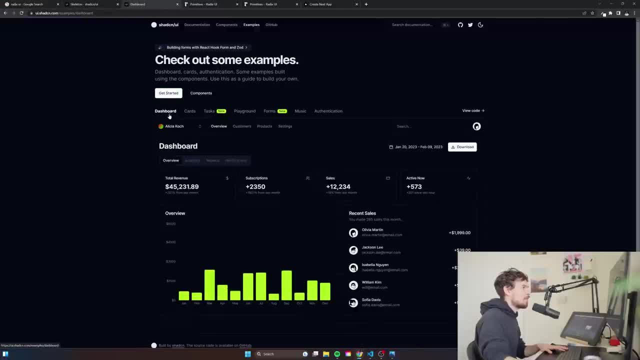 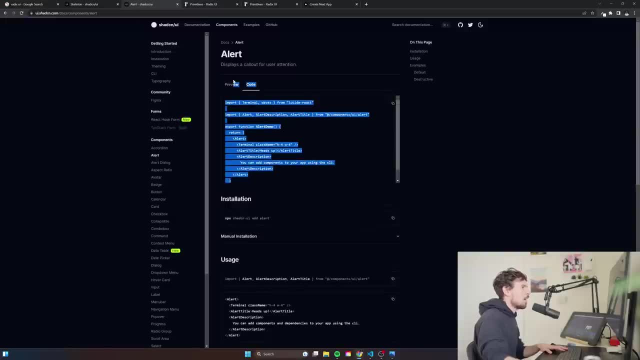 for you to just go here, find a specific uh UI component, maybe, let's see, maybe the alert here right And you can just copy paste the code and that's it. But now they have a CLI, which is really cool, Uh, so you can just pop in and 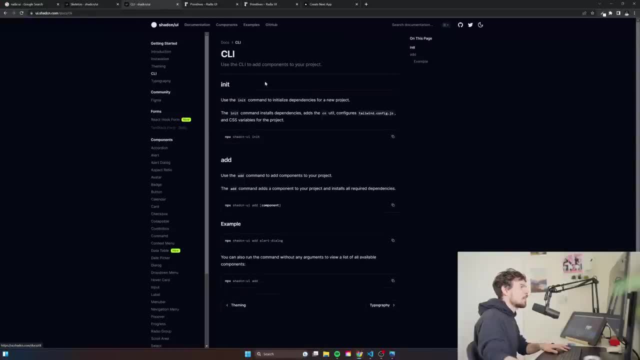 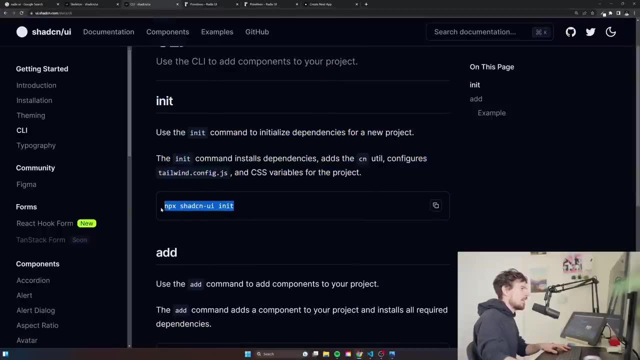 install that specific component that you need. So if we head over here to the CLI, you can run this command here called MPX, chat, CDN, UI and net. All right, So if we run this- I already ran this, Uh- and if you have, 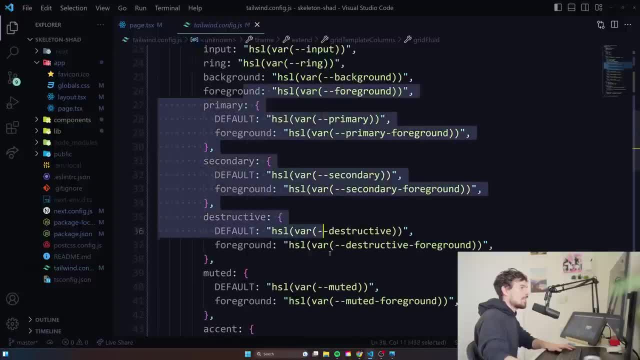 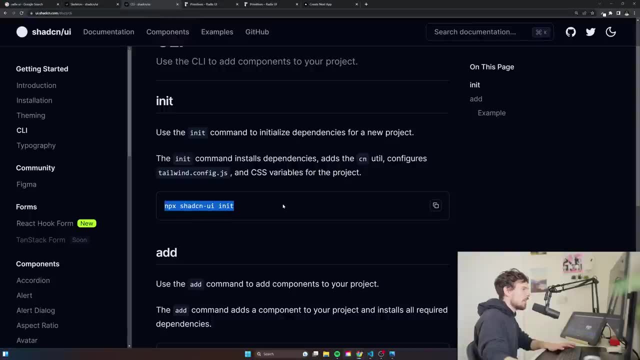 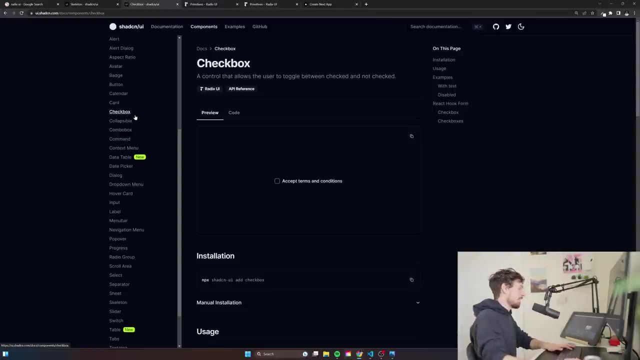 tailwind as well, installed, um, it's going to add all the necessary configuration to it, should I say All right? So after we run this, perfect, now we can just head down to any component that we want to use, And I may make a video. Let me know if you want to see a more. 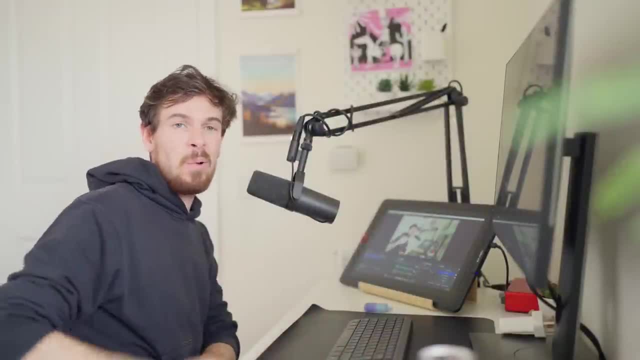 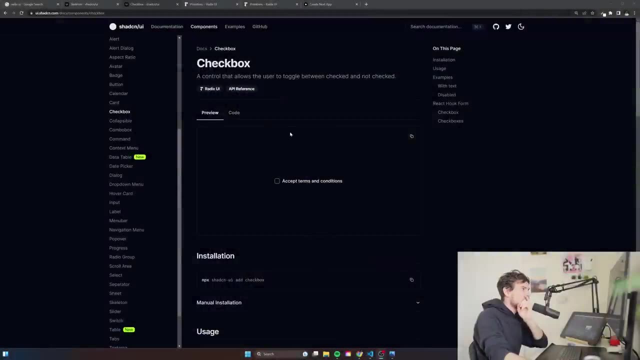 in-depth video on chat CDN. maybe we can build out like a whole whole app with it. That'd be quite fun actually. Um, but yeah, let's head over back here And we're going to search for skeleton. So here we go. All we need to do is run this command: MPX. 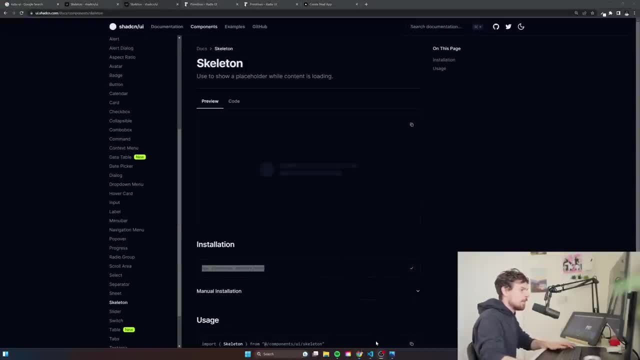 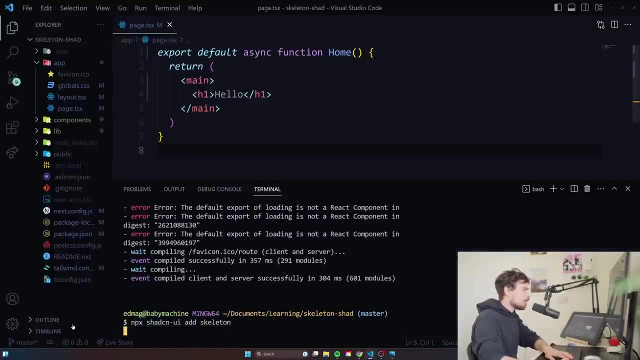 chat CDN at skeleton. I'm going to use MPM for that And I think I already did it. once you install it, So once you add it like that, it's going to create a oops. let me close that up. Uh, it's. 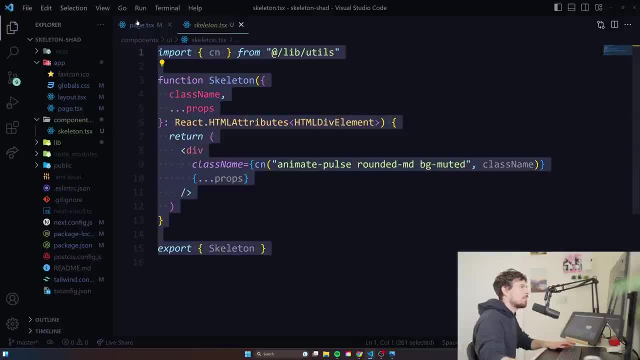 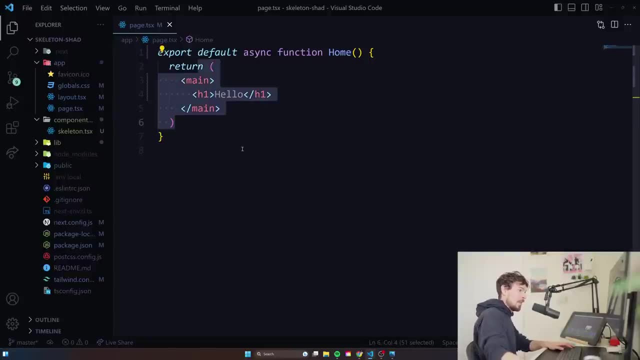 going to create a component here for you automatically, just like that Super cool. Okay, So let's actually create something here, Because we have absolutely nothing now And that's the present. So what we're going to do is, yeah, Fetch some games. So I'm using ROG RAR API for fetching games, Uh, so all we can do is just: 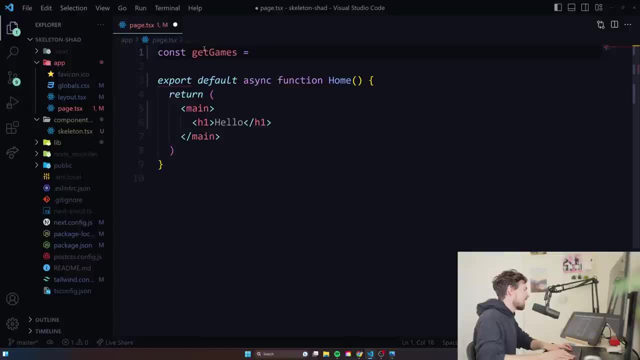 do a const get games here. I said that equal to an async function, like that Cool. And then, and here we can say const response, And here we are going to. we're going to do a const response, And here we are going to do a const response. And here we are. 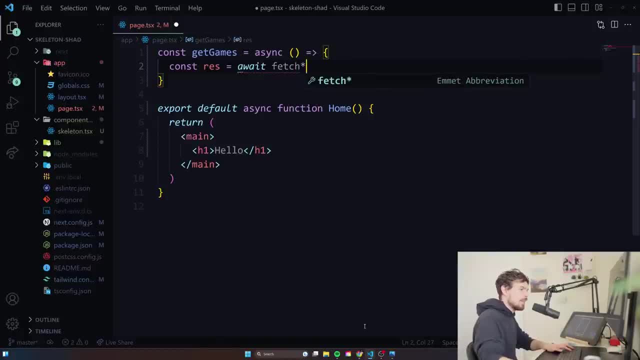 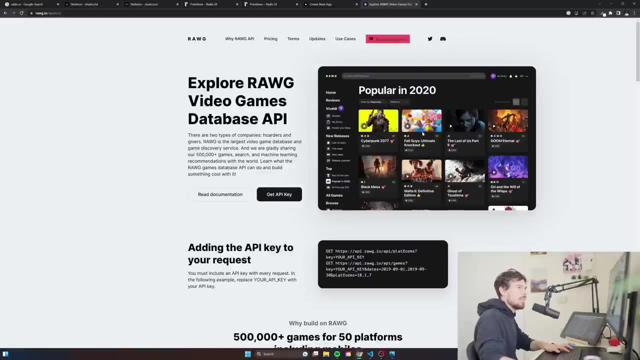 going to do a fetch request. So again, I'm using- let's see where is it- Rogue API. All right, And yeah, you can fetch any games. You can fetch popular games type games like Redfall, uh. 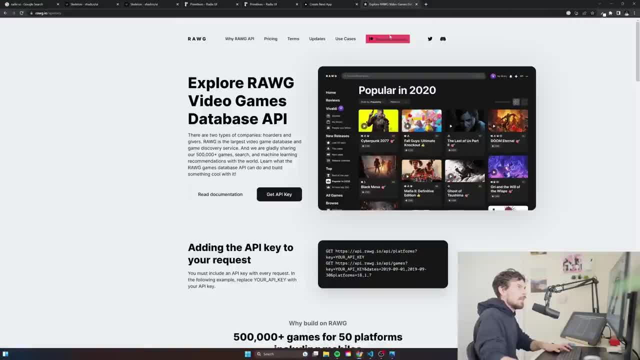 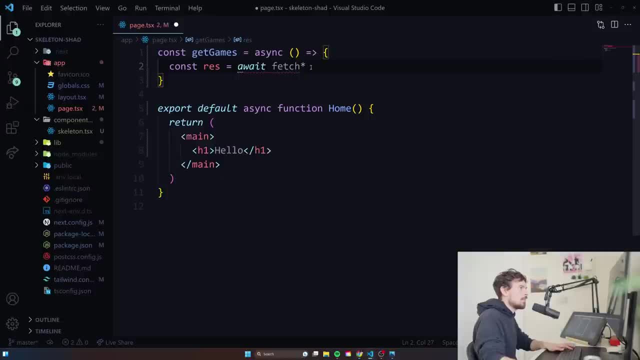 really good games like Zelda, Um, but yeah, you just get your API key, you add it in here and then you fetch the game. So let's do that, Await fetch And the link to this is going to be in the. this is going to be HTTPS, like that. Let me see here APIrogio, slash API, slash games, And then 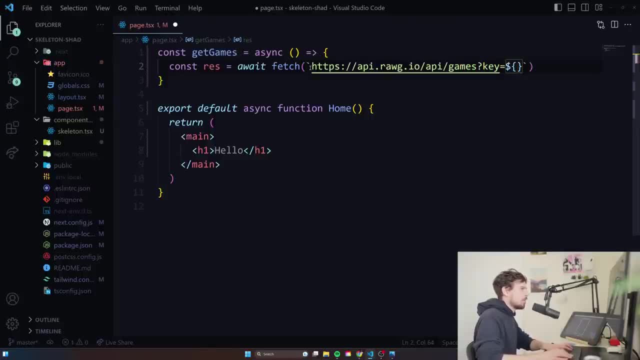 here I can add my key, which I just added to my uh EMV local here. All right, So that's where my API key lies, So I can just add it with process EMVrog like that. Cool, Now I can check if the 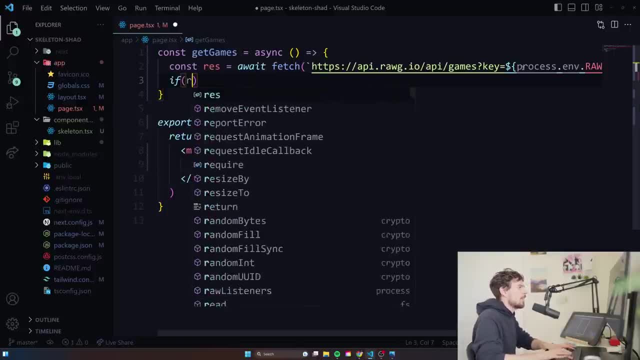 response is not okay, So I can just add it with process EMVrog Like that. Cool, Now I can check if the response is not okay. So I can say if res is not okay, That means I have some sort of error. 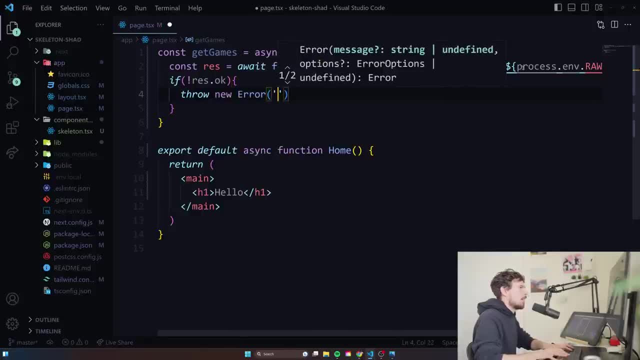 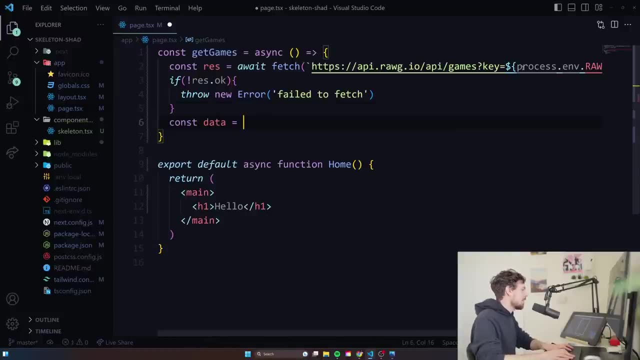 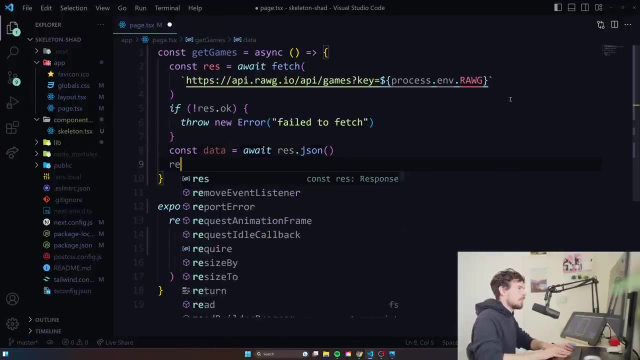 So I can just throw a new error and say, uh, failed to fetch. But if everything is okay, I can say cons, data is equal to await resjson, like that, All right, And I need to return this. I'm going to say return data, like that. I guess you could do it in one line, but 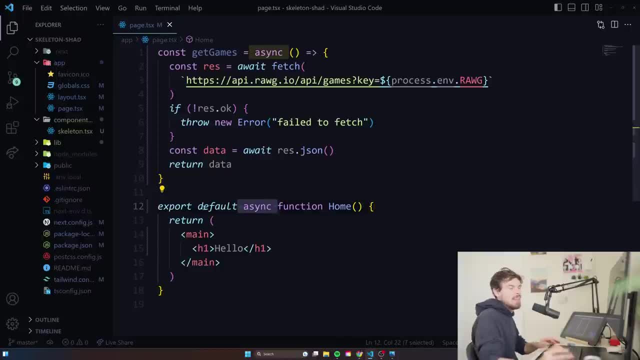 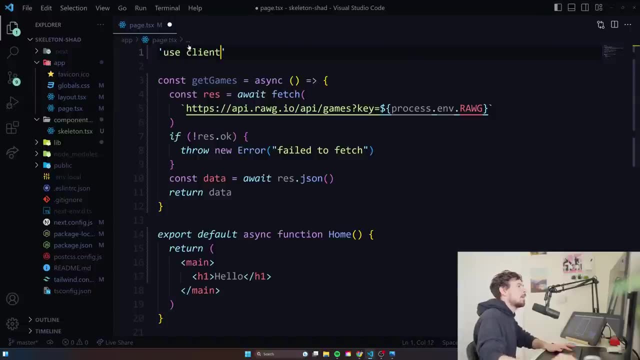 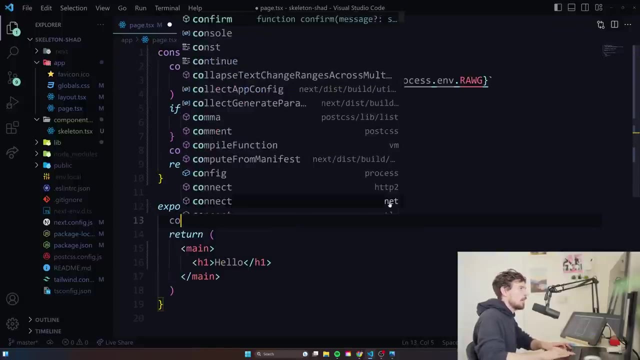 it is what it is. Okay. So now here: uh, this is a server component, right? If you don't have use client at the top here, that means you're working in a server component. Um, so what we can do here is just say: const games equals, get games like that. 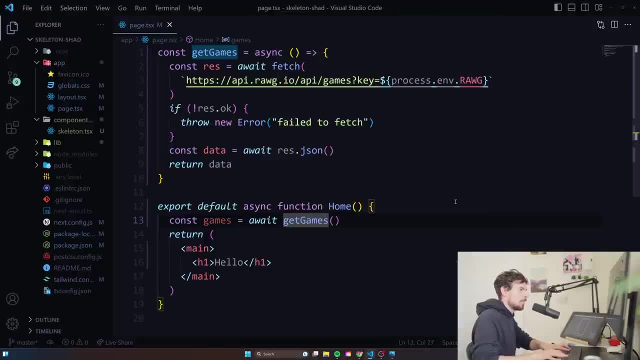 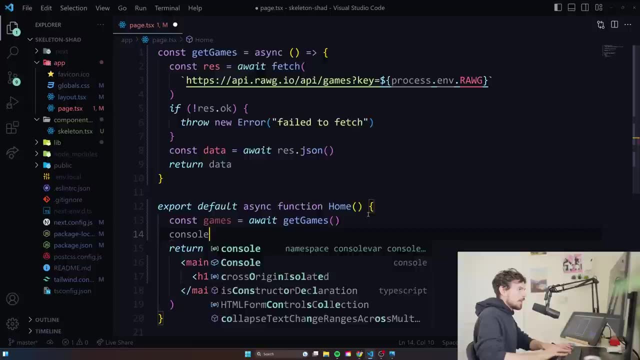 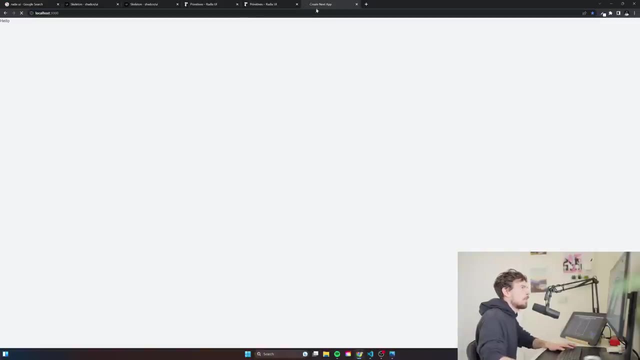 And we have to add the weight as well. Like that, Perfect, All right, So I remember this is an in component here. Uh, and let's, let's see if that works. We're going to console log out games. have a look here and try to visit the local host 3000.. So we can actually see if we can fetch that. 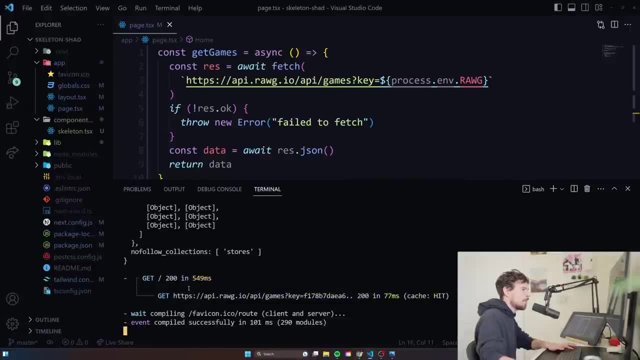 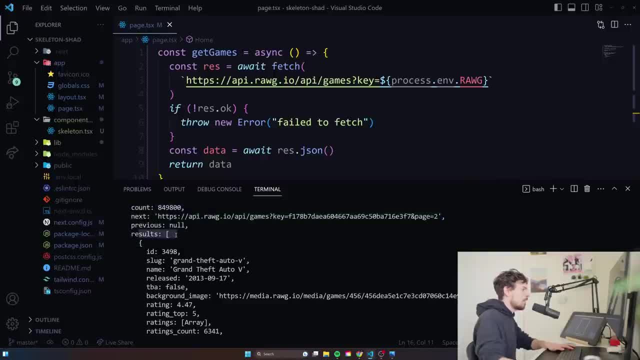 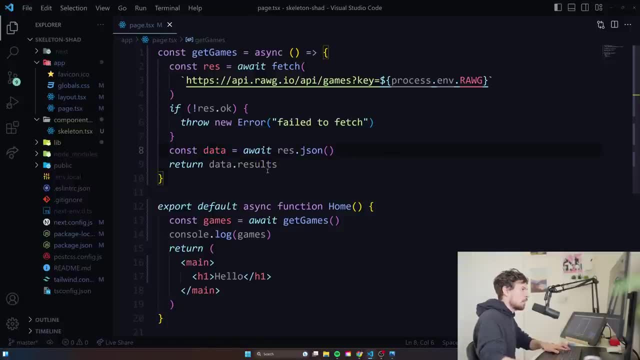 object, As you can see, and you have counts- next previous and results. Now, results is the array that actually holds all the games. So I'm going to return that data, dot results, and I'm not going to take everything out, So I'm only going to pull a couple of things out here in my types. 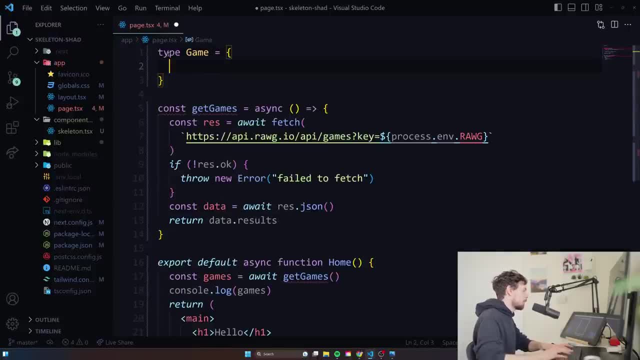 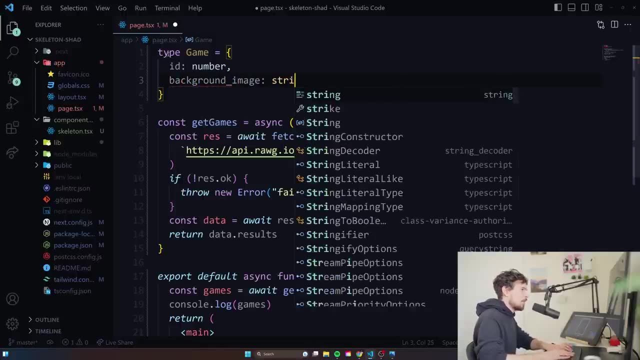 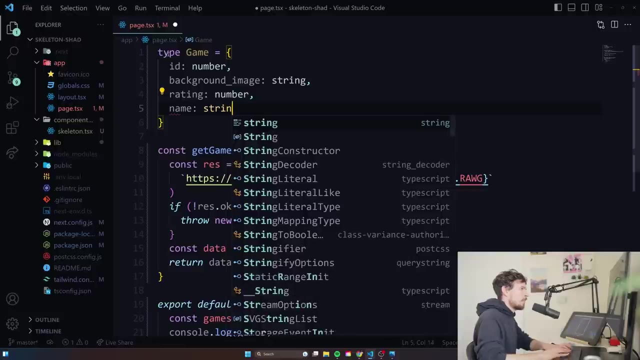 So I'm going to say type game equals to. I'll just pass in the ID. We'll do a background uh image, which is going to be a type string. We're going to do a rating, which is a type of number and a name. That's a type of string. Again, all I did was literally. 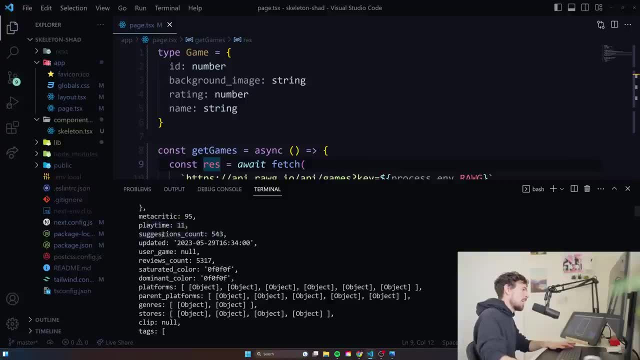 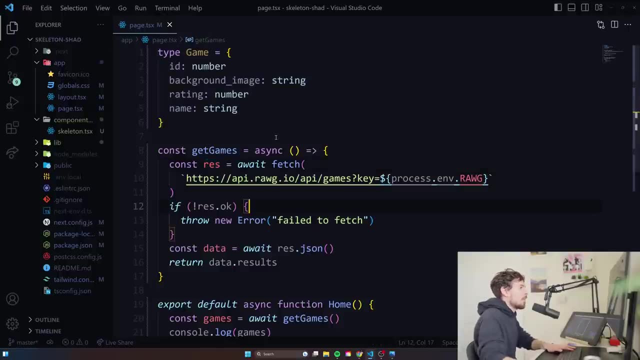 go through all of this shite and I pulled out the uh necessary properties that I want to use in my app. So in this case I'll just use these four. Um, all right, And the way we can add it is here in the get games can add a colon and say promise and add this as a generic right. 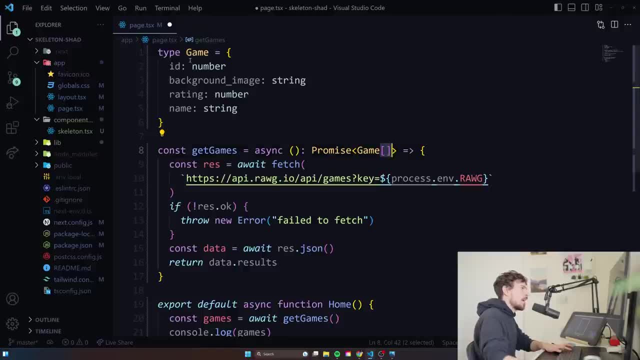 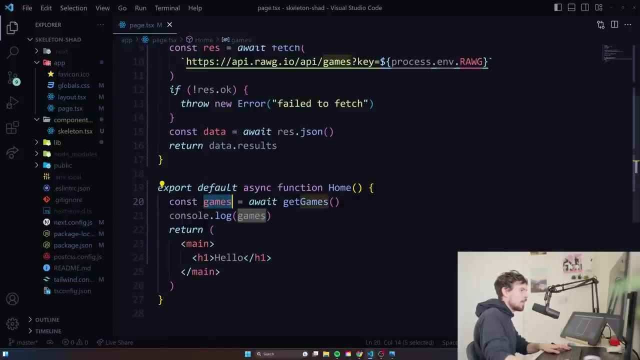 here, But we want to make sure we also add an array Um, because we have multiple ones. right, We have an array of game objects, So we pass that in there And, as you can see now um type script works on my games down here. So if I do games, 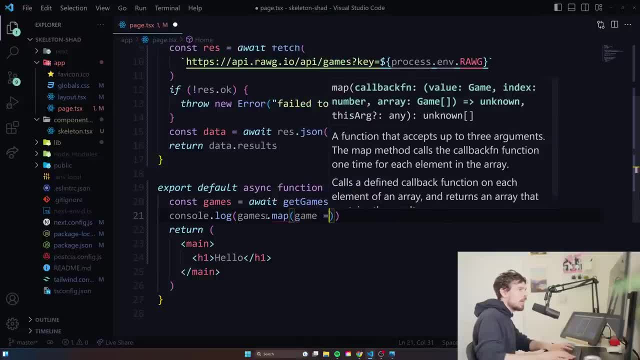 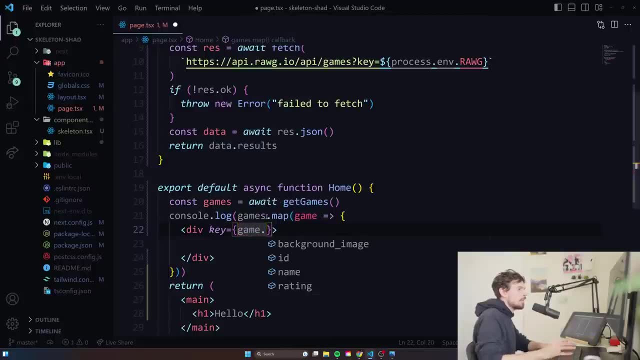 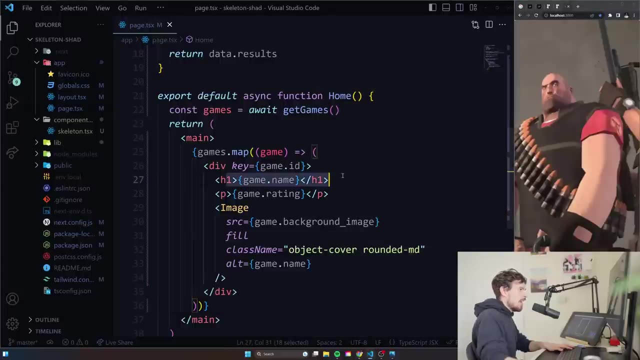 dot, uh, map over each game. like that I can return a diff, for example, uh, with a key of game dot, And look at that, We have the auto completes on return game ID There. Okay, cool. So I added the H one here saying game name, the P tag and the image. Now 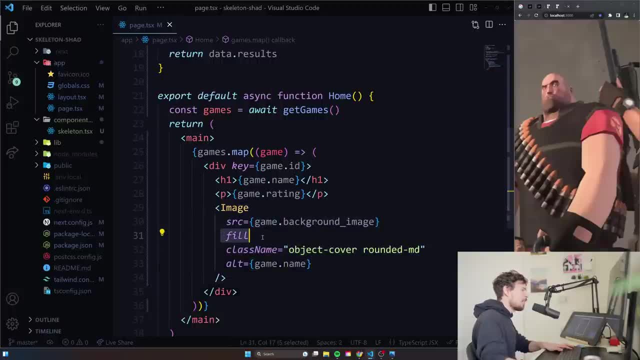 the way I like to work with the image tag is to just add a fill on it And then I can customize everything else with the class name. So by default, fill is literally going to just take up all the space- uh, relative to the outer diff that it has. So if I wrap this in a diff like that, 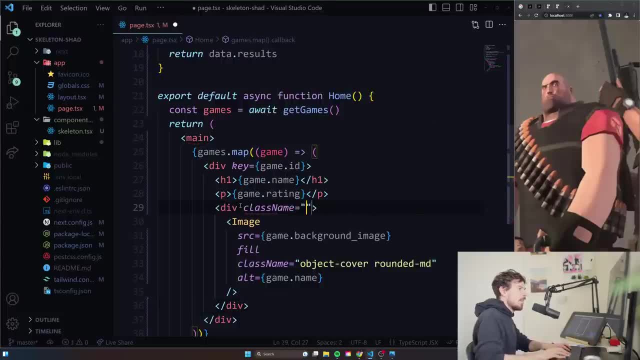 and I can go here and add a class name to this and say I want it to have an aspect of video which is 16 by nine, and I can add a relative. So size this according to that. And there we go. Look at that, We have a nice. 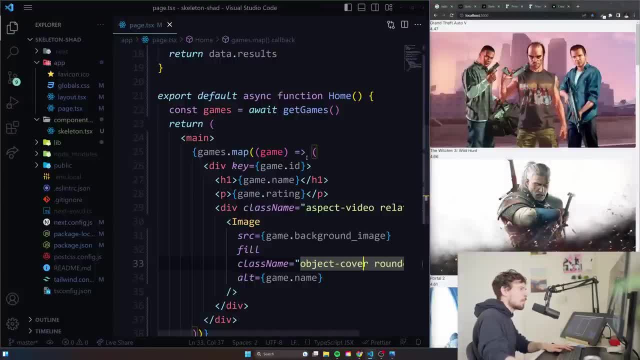 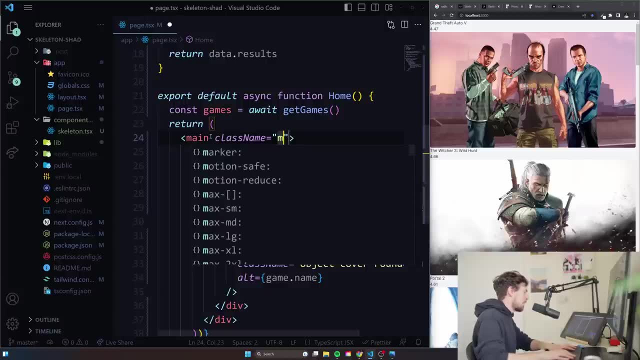 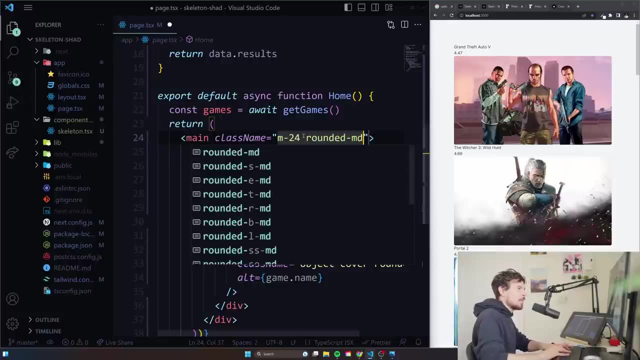 system here going. It's not like responsive or anything, but we can quickly make that. I'm going to go to the main tag here and I'm going to start off by just adding some margins: M 24.. There we go. Just so it's not all stuck up there, I can add a rounded MD. 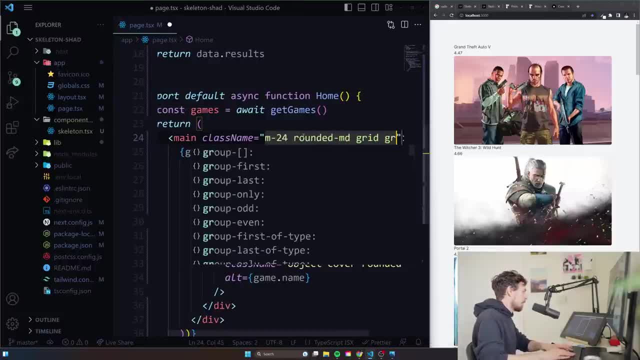 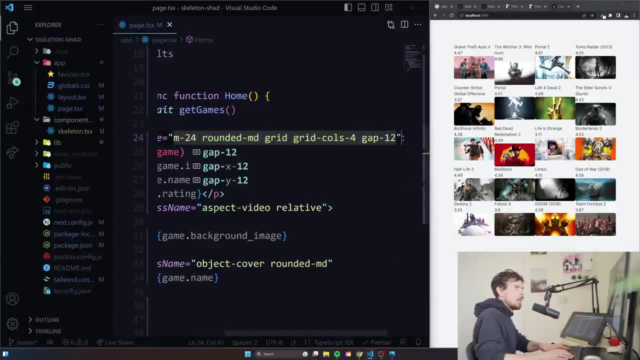 and then we're going to do a grid. All right, I'm going to say: grid calls four. There we go. So we have four columns now, and I'm also going to add a gap of 12, like that. Cool, Perfect, Now what I'm. 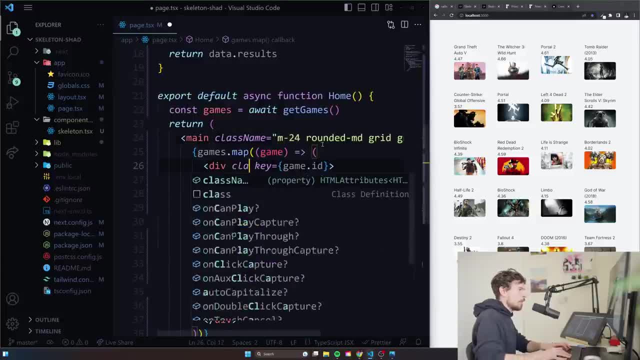 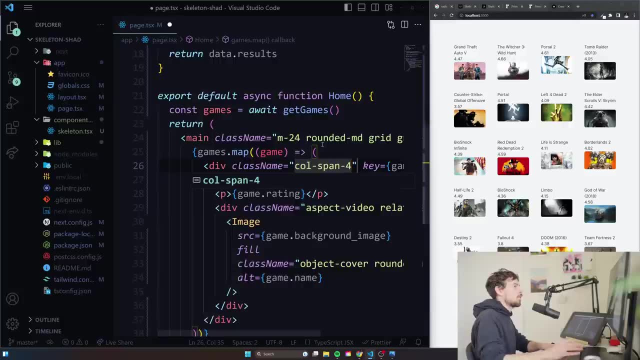 going to do on this inner diff here where I'm looping over, I'm going to add a class name to this as well And I'm going to say Cole span four. So how, how much should this div span across these columns? Cause, remember, we have four columns. So I'm saying stretch from one to. 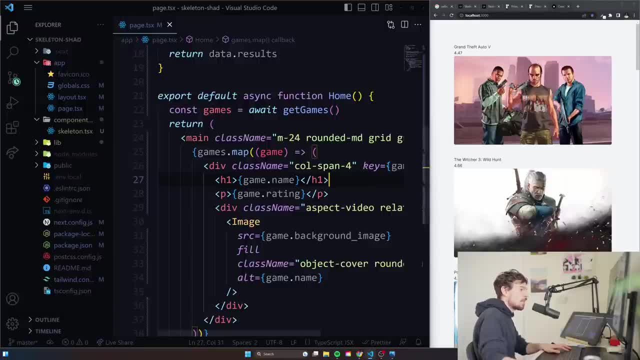 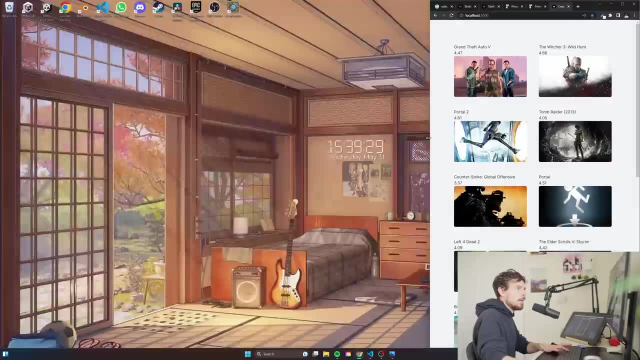 four and head safe. So that means it's taking up all the space. Now if we go on larger screens I can say Cole span should be two. So there we go. So if I go really small it's going to go to. 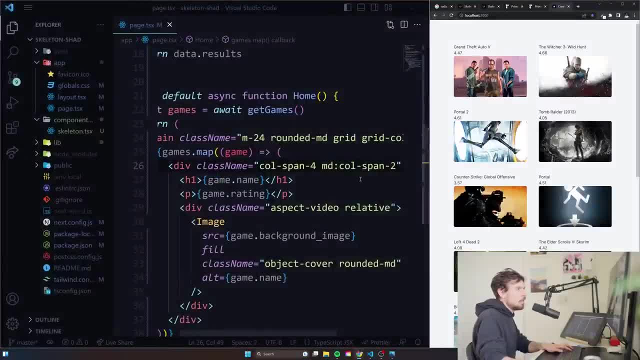 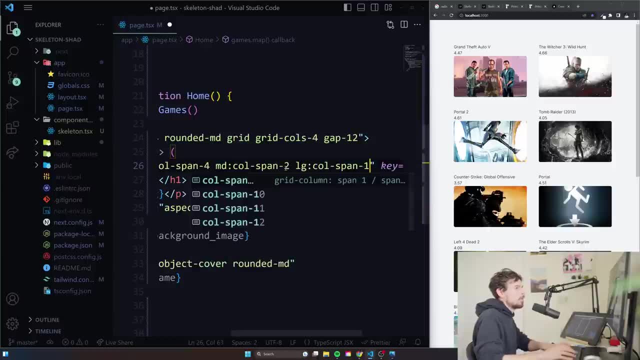 one. If I go bigger, it's going to go to two. Now you can keep going like this If you want. if you want to do an on large screens, I want a Cole span of one right. So then you would have. 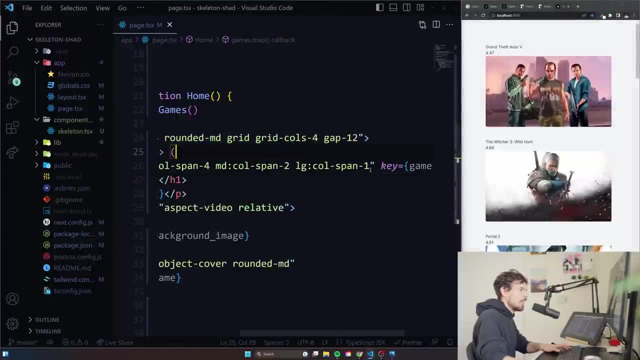 to keep going like this. So I'm going to keep going like this, So I'm going to keep going like this. There we go. No, I probably don't want that. That doesn't look too good, So I'm just going to get. 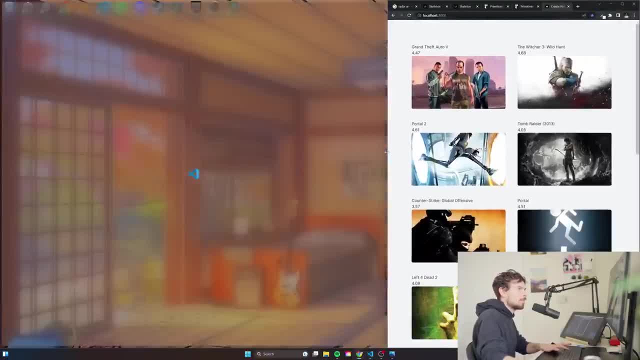 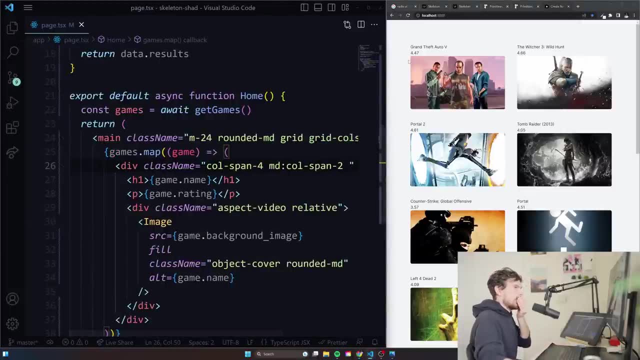 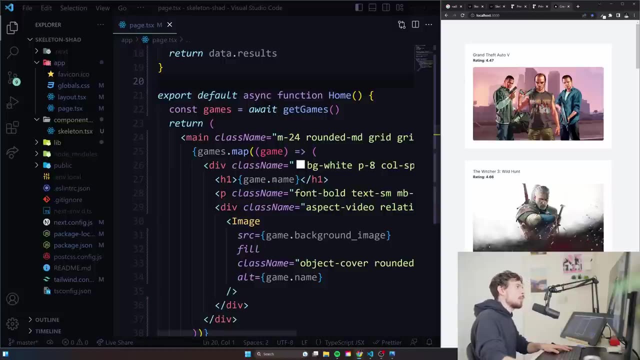 rid of that and keep four. There we go Two. Sorry, Okay, cool. So we got that going for us, which is nice. Yeah, You could style up the text and everything, but I'm not going to waste your time with that. So how can we do this? What if I go up here and I say something like await new. 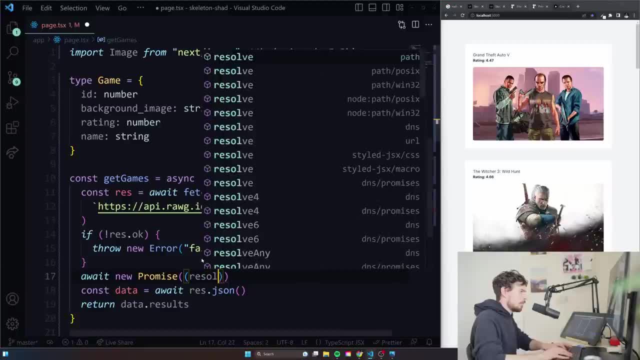 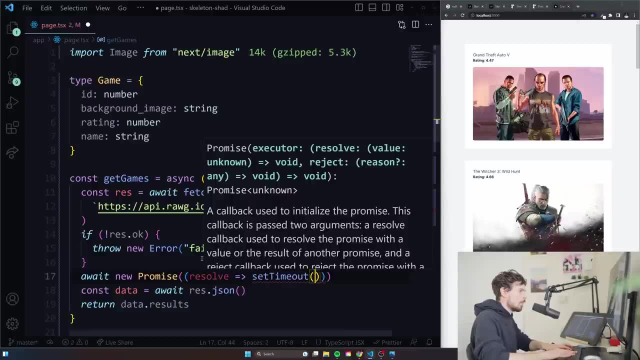 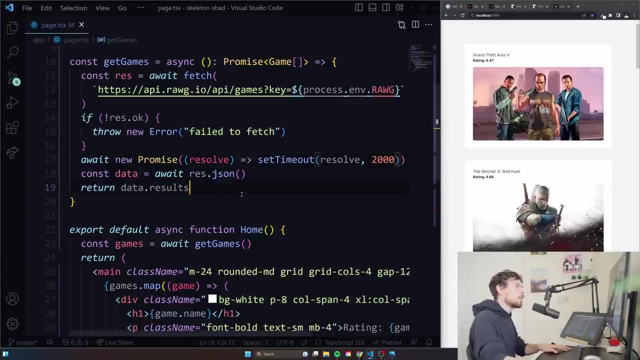 and we'll have a resolve here like that. I'm going to say set timeout, set timeout to resolve and 2000.. All right, What does this code do? So, essentially, we're awaiting and creating a promise and we're resolving the promise in the same line of code And basically we're adding a delay with. 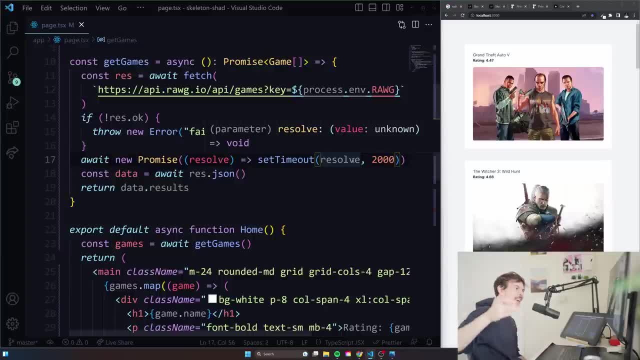 the timeout. So we're saying, as long as the set timeout is running, basically stop this from finishing, wait for this promise to resolve And when it resolves, keep going and fetch the data. So in our case, it's going to take two seconds for this promise to be resolved. So if we refresh the 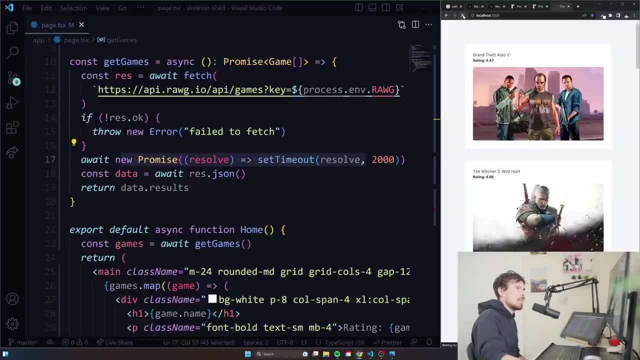 page now. um, I guess we'd have to close this and go back. Uh, you're going to get a blank page for two seconds, right, And you don't want that when your data is loading. So how can we transform this? 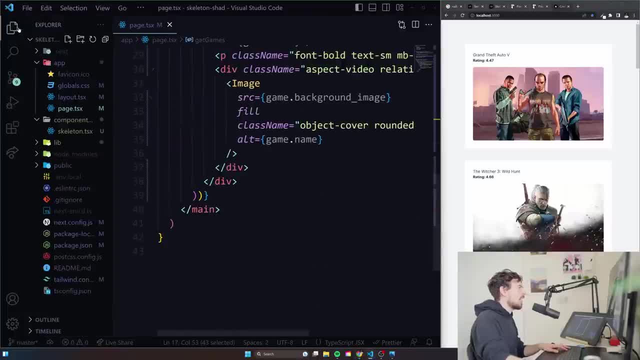 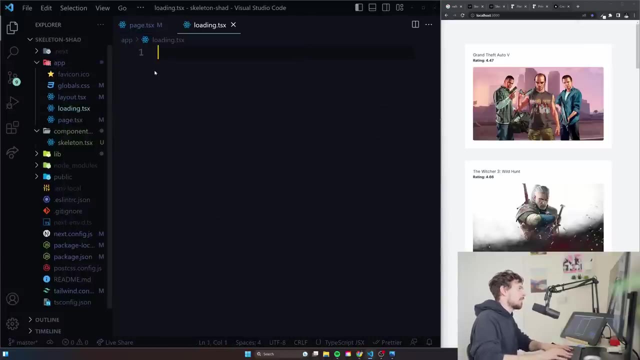 and create a skeleton, super easy. and next 13,. what you can do is just go to the page um or the folder where you have the page, and create a loading the TSX, Okay, cool. And then when we can do is say: imports, sorry. 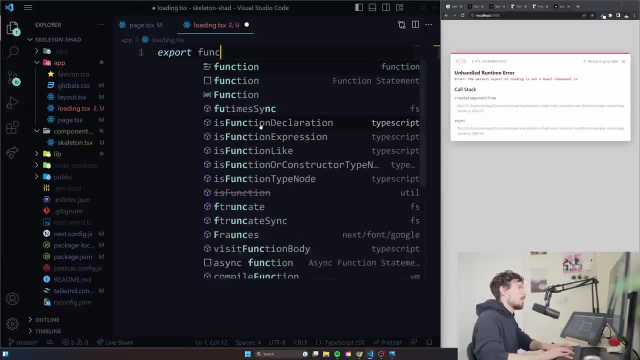 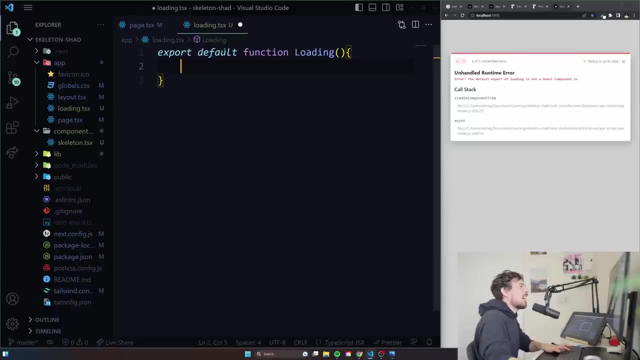 export function default. I always get these wrong, Do you? Oh my God, I find that impossible. I always do export function default, or I don't even know how I do it. Sometimes I start doing const. It doesn't matter who cares, Let's try to return something. So here I can just pretty much. 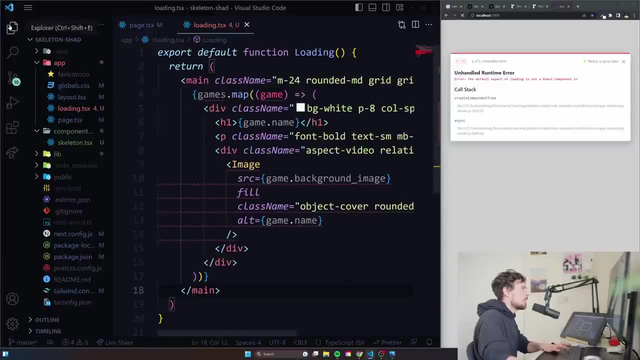 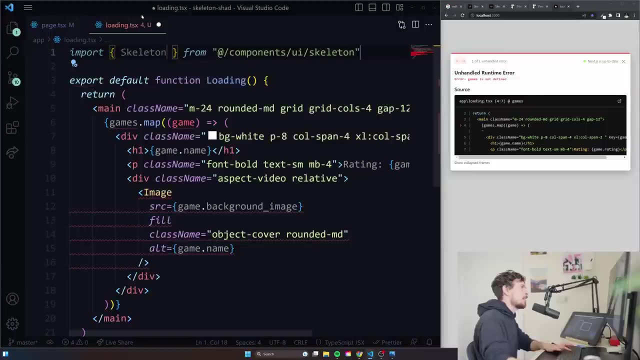 copy paste this over like that And I just need to Make a couple of we changes. So first of all, we need to import, uh, that skeleton that we got from chat, save the end. So there we go, Import skeleton like that, And since we don't have any, what you? 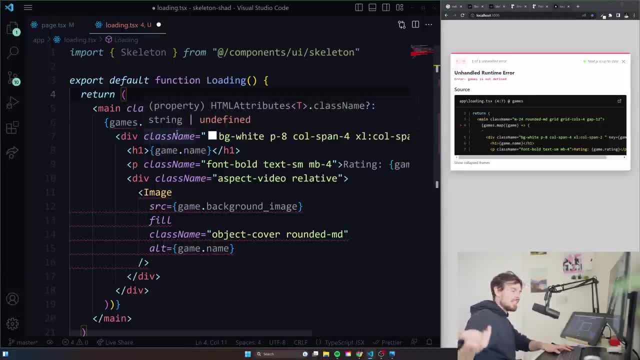 call games here. right, We're not fetching any data and we don't want to fetch data, because that's the whole point. We're trying to stop and show something else: was the data is fetching. So what we can do is do something quite fun here. We can say array and we can say from: 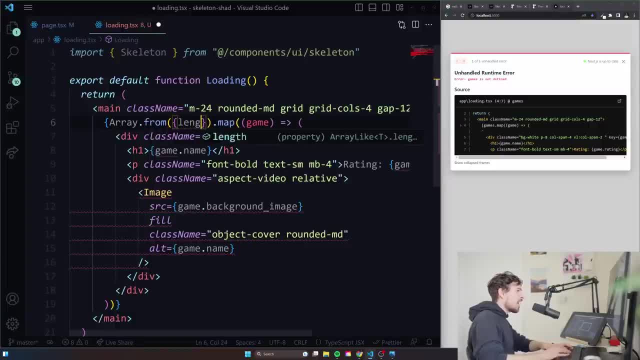 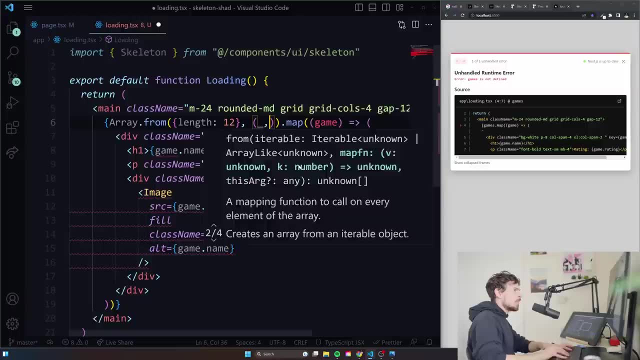 and I'm going to say here: length in an object of 12. All, right, And then after this object I'm going to add the comma and do an underscore and an I, and then I'm going to run a function here like this: Oops, like that, Okay, I'm going to say I plus one, and then we can map over it. 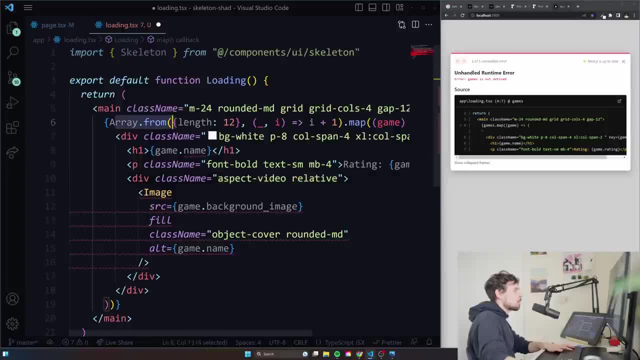 the same way. So essentially what I'm doing here is just getting an array from scratch and I'm getting the index and I'm adding a one to that index, And then here I'm just going to say ID. It doesn't really matter what I add here, I just 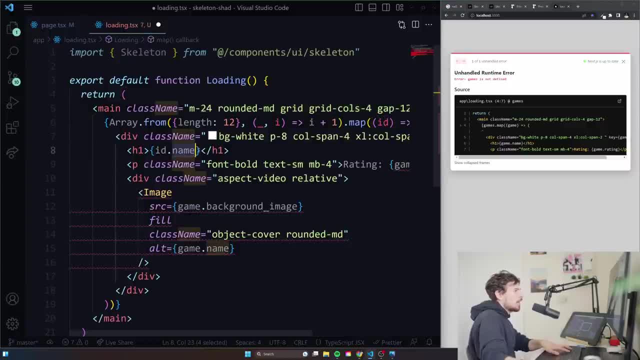 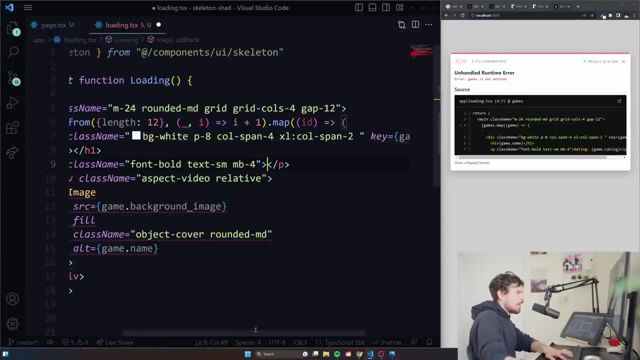 want to make sure I can loop over it like 12 times. Uh, here we can leave this empty. That's fine. I'm going to get rid of this as well, because we're not going to add any HTML here. We're just going to control everything with the styling and the image can go as well. 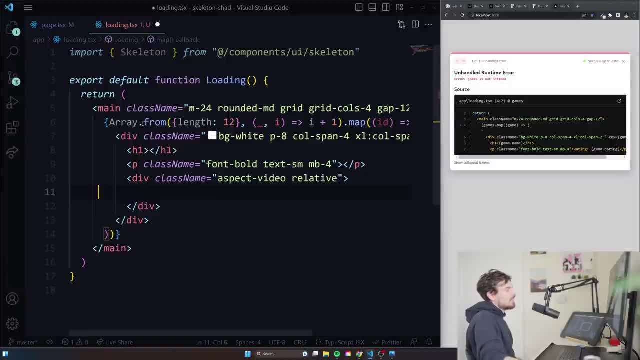 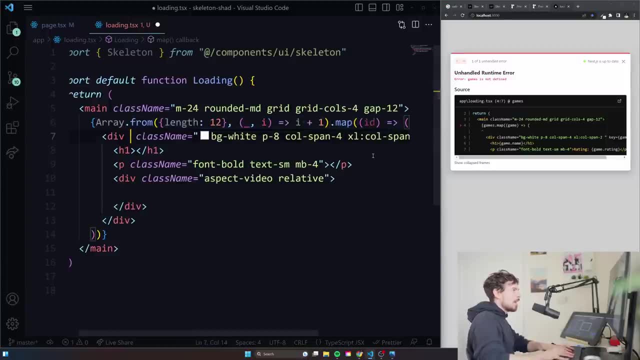 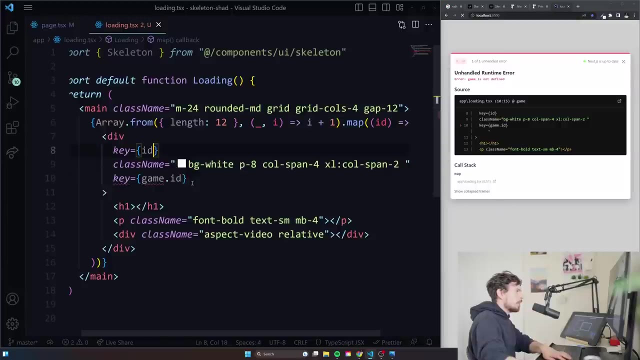 All right. so again, I'm just, yeah, creating an array from scratch. here I'm looping over it, and then here I guess I should add the key. I'm just gonna pop an ID here for now. that's fine. 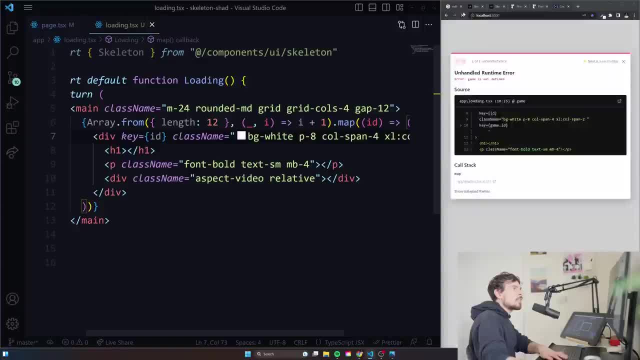 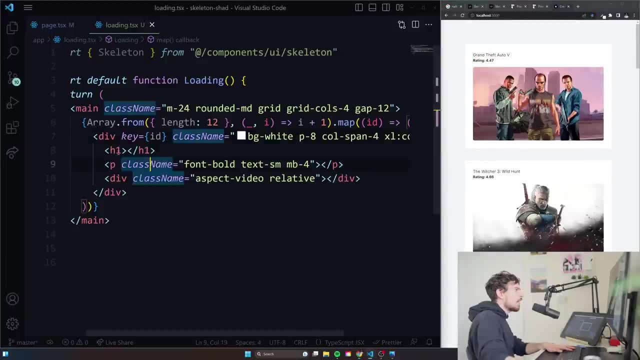 Let's get rid of this old one And let's see what other errors we have, And it looks like we don't. so, as you can see, we just have this flashing white screen now, and then we get our text back. So, rather than doing a H1 here, 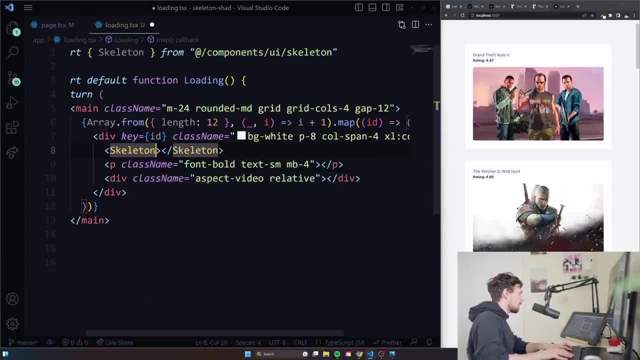 what we can do is say skeleton instead, like that, And here I can add a class name to it and I'm just gonna add a bit of height to it. So I'm gonna say height is gonna be six and the width is gonna be, let's say, half of this card. 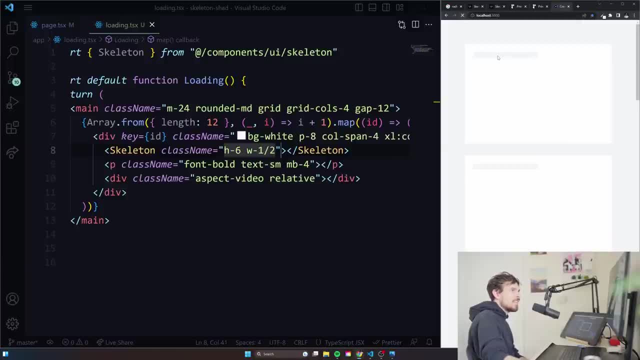 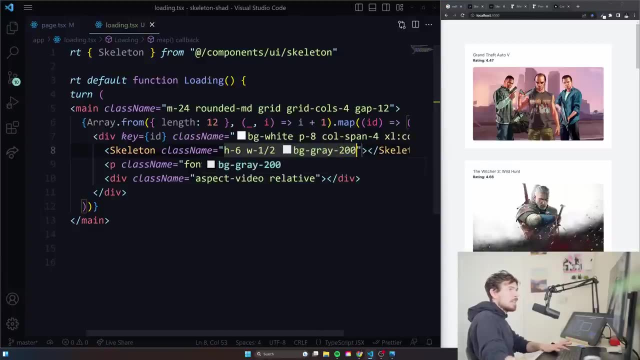 Now if we refresh, look at that. we are getting a nice loading animation right there. Now, if it's hard to see, feel free to customize it. You can do a BG gray of 200 on it, hit save and look at that. 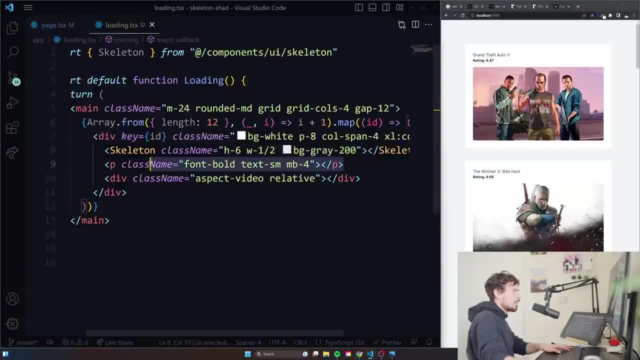 Look at that cool, So I can do the same thing basically for the paragraph here. Let's turn this into a skeleton And rather than doing this, I can still keep the margin bottom. I guess I could do a margin bottom of like two at the top as well. 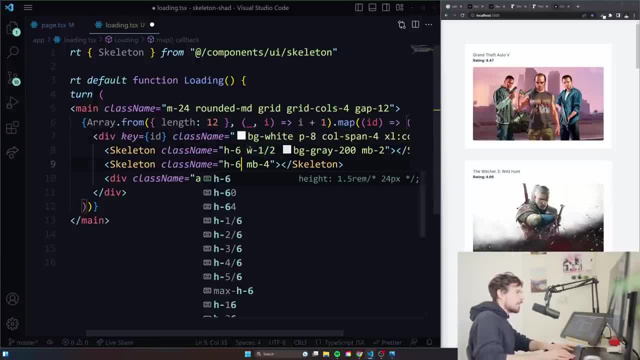 And then here all I need to do is, again, I can do a height of six or whatever you prefer, width of maybe a quarter of that, because it's really small, And let's refresh. and there we go. How cool is that. 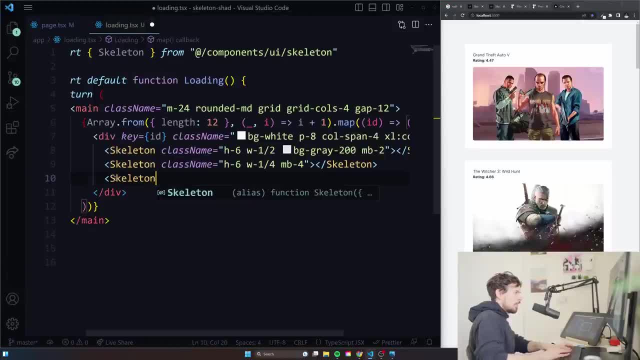 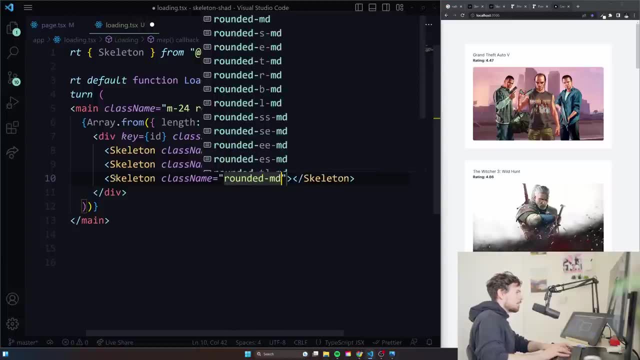 Finally, for the video. again, I can just make a new skeleton here from scratch, to be honest, and just add a class name to this and do maybe like a rounded of medium I think I had on it. Width is gonna be full. 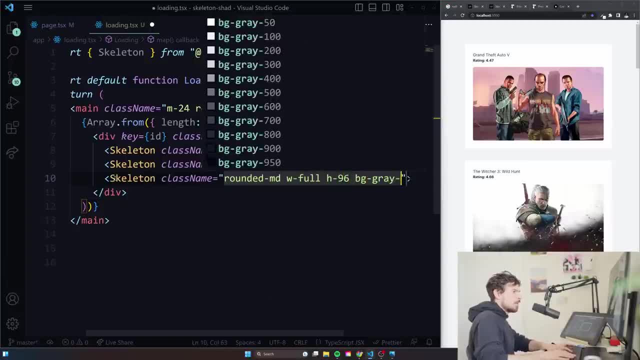 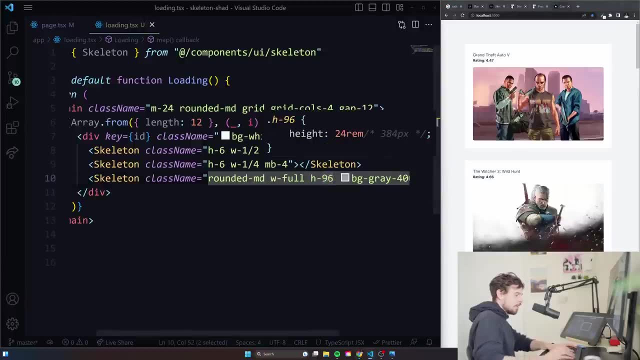 I'm gonna add a large height to it and a background. Let's do something else like 400.. And do a refresh and take a look at that. That's pretty cool. Maybe that's a bit too big. Maybe you do it in a more responsive fashion. 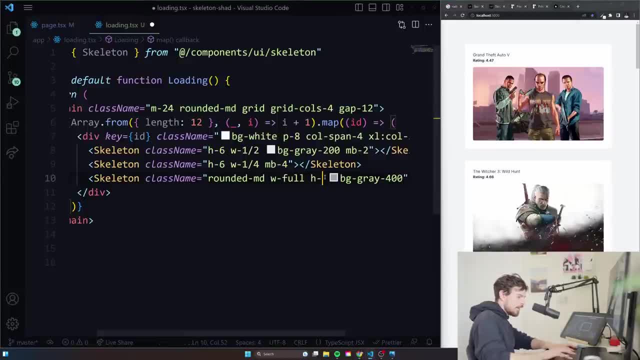 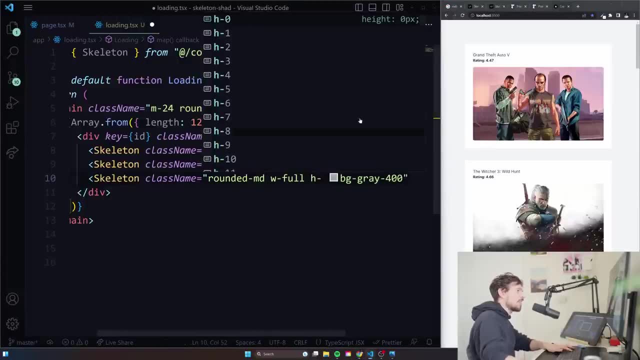 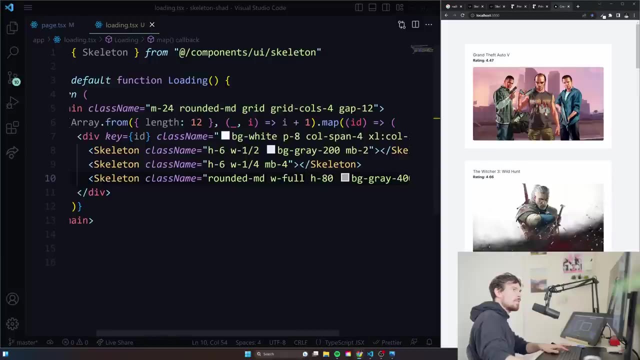 and a hard-coded like that. Oh, That's not working. Height: 80,, four And hit save- That is weird. H. why is that not working? 80, that's gonna work. And there we go. Look at that boom. 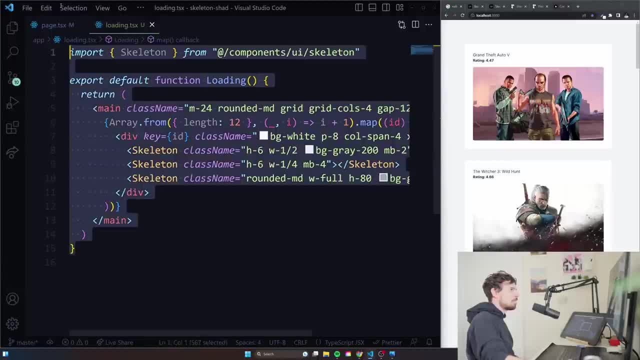 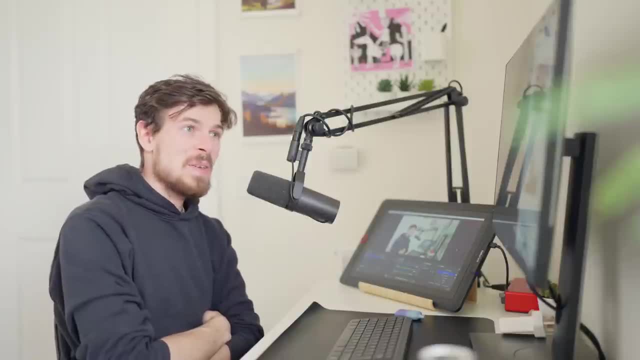 How cool is that? So we added a full-on skeleton and barely any lines of code. Yeah, I like that. That's really cool. All right, so that's gonna be it for me. Hope you enjoyed this. Let me know what you think of chat CDN. 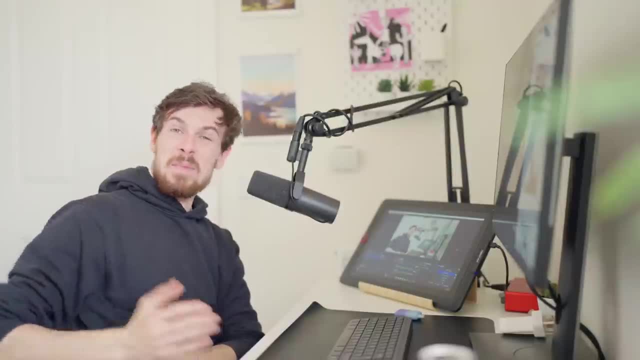 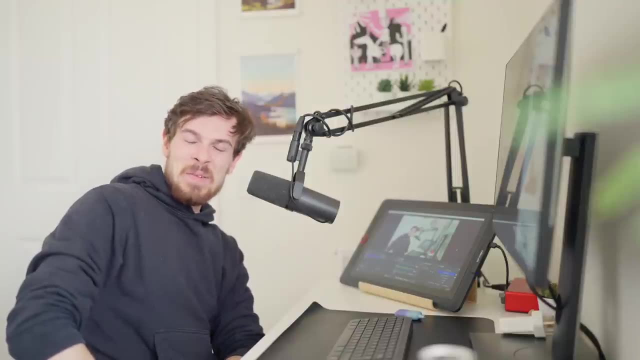 CN. CN not CDN. Have you played with it? Do you like it? Do you have fun with it? Hopefully in a non-weird way, And yeah, that's gonna be it for me. Please drop a subscribe if you enjoy the content. 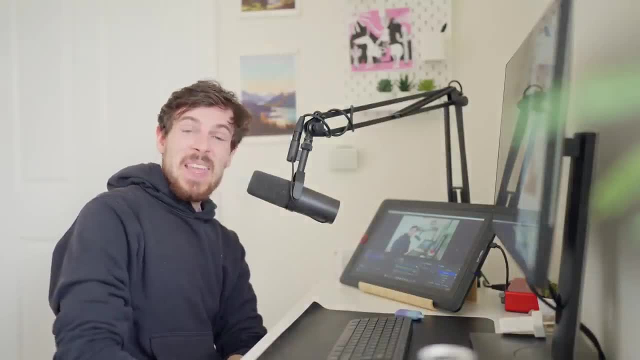 on this channel. I'd really appreciate it. And yeah, I'll see you in the next one. I have loads of exciting things coming up. I'm doing the Astro project next And, I'm not gonna lie, I've been working a lot.